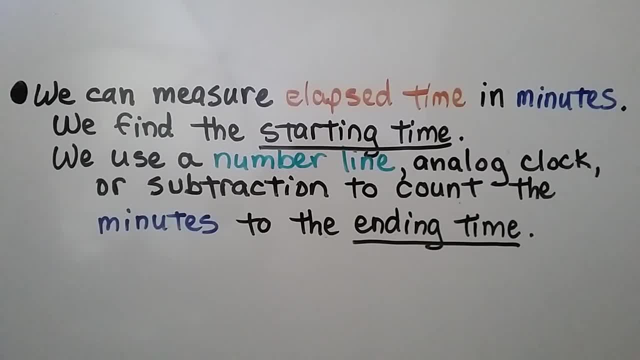 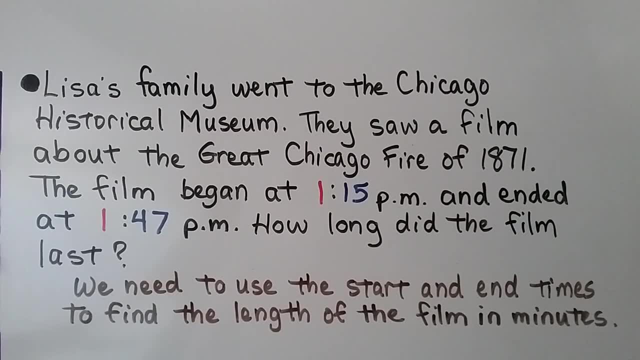 analog clock or subtraction to count the minutes to the ending time. Lisa's family went to the Chicago Historical Museum. They saw a film about the great Chicago Fire of 1871. The film began at 1: 15 pm and ended at 9: 9 pm. 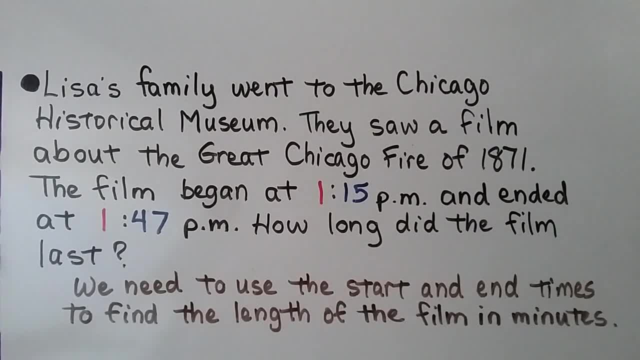 Lise's family went to the Chicago Historical Museum and they saw a film about the great Chicago fire of 1871. The film began at 1: 15 pm and ended at 9: 8 pm. at 1: 47 pm. How long did the film last? We need to use the start and end times to find the length. 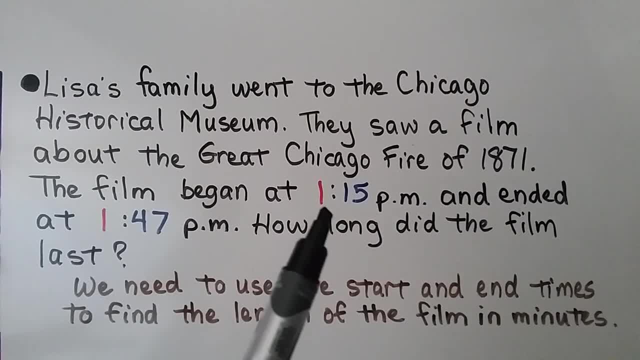 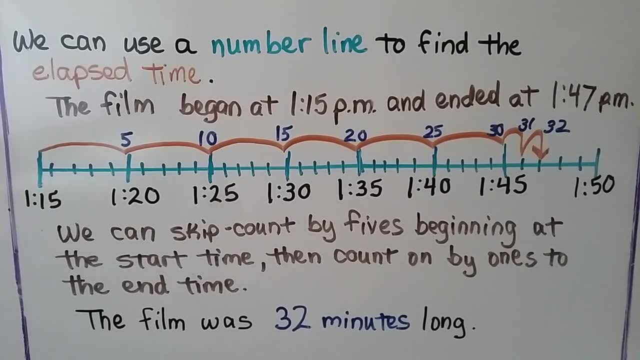 of the film in minutes We see it started at 1: 15 pm. It ended at 1: 47 pm. We can use a number line to find the elapsed time. We can skip, count by fives, beginning at the start time, then count. 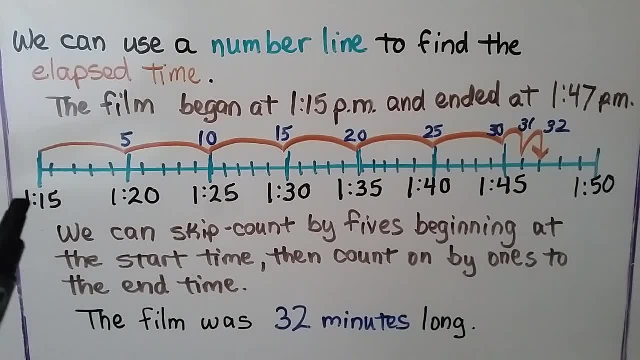 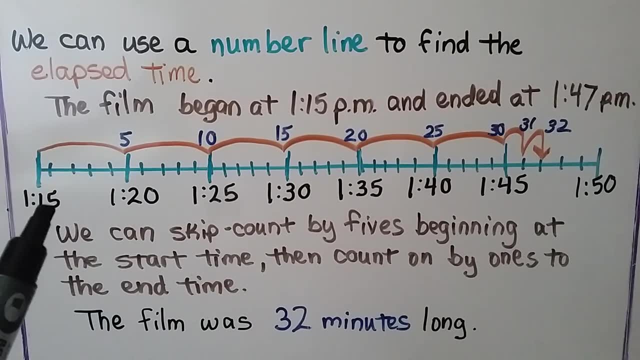 on by ones to the end time. Our number line starts at 1- 15 when the film began, and because it's a 15, we can skip count by fives, can't we? And our number line can show 1- 20,, 1 25,, 1- 30,. 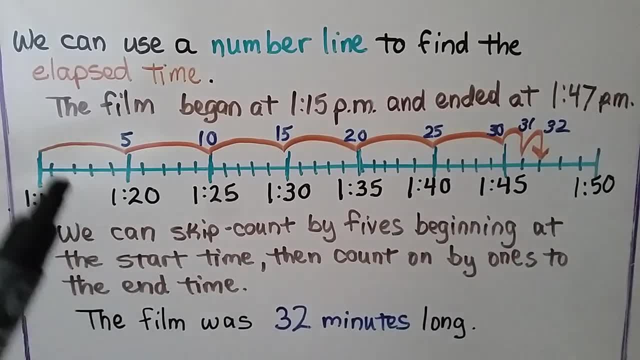 1, 35,, 1 40,, 1 45,, 1 50.. We skip count 5, 10, 15, 20, 25, 30 minutes. We need to get to 1, 47, so we're going to count on one minute increments at a time. we get to 31, 32, so the film was 32 minutes long. 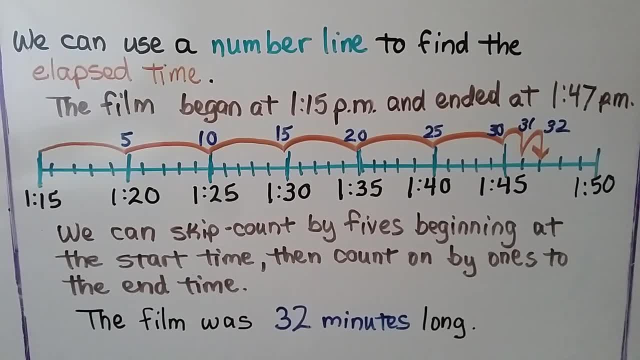 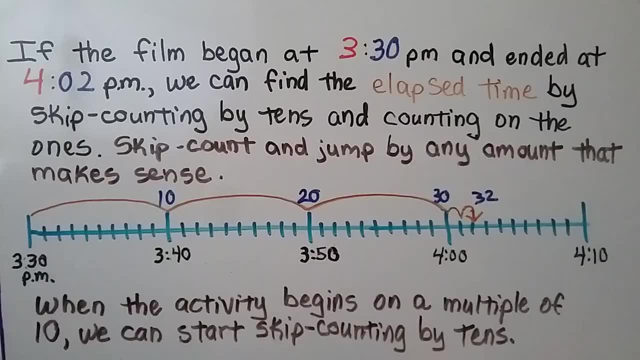 We skip counted by fives, then we counted on by ones until we got to the end time. If the film began at 3: 30 pm and ended at 4: 02 pm, we can find the elapsed time by skip counting. 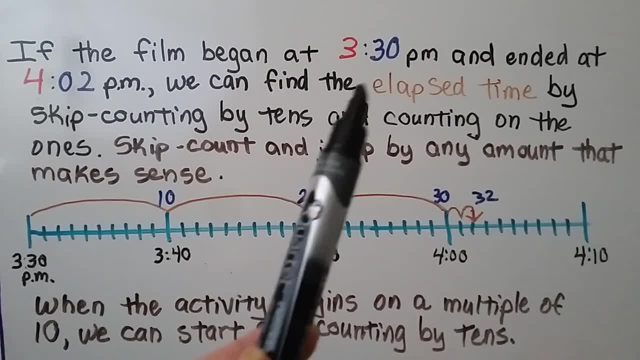 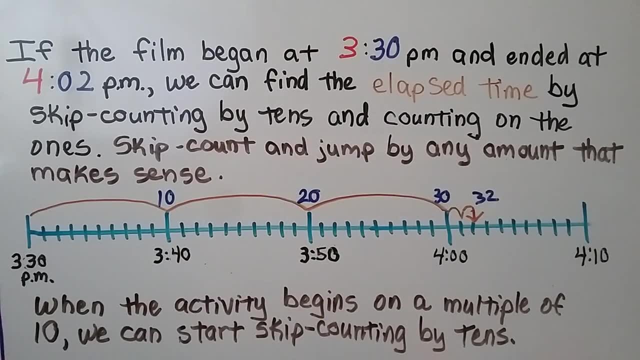 by the five steps. We have these numbers, one by 2, some west, some west west and others by the 10s and counting on the ones, because this is a multiple of 10, like 10, 20, 30, we can skip- count by 10s and then we'll count on to the end by ones. so we start. 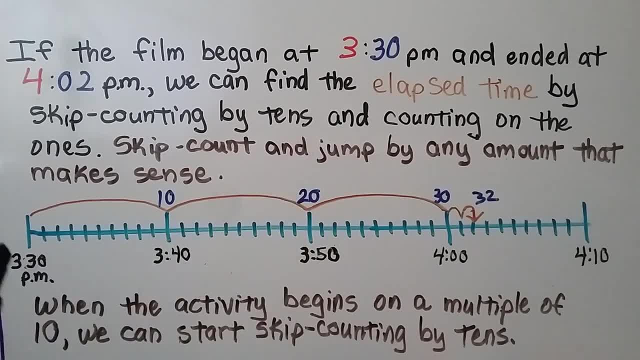 at 3: 30 on our number line. that's the time it started and our number line is going to go to 3, 40, 350. then it'll be 4 o'clock, then it will be 4- 10. so now we can skip count 10, 20, 30. we're at 4 o'clock, but we need to go to 4 o 2, so we 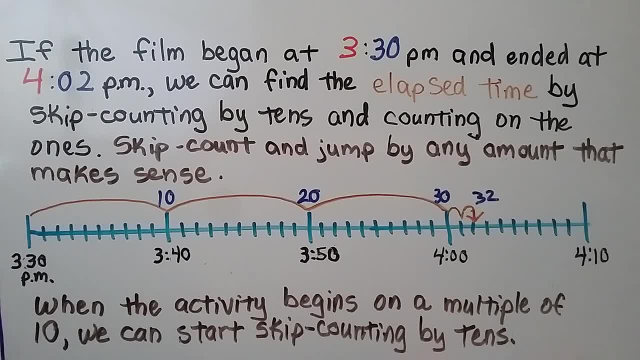 go 1, 2, that puts us at 32. when the activity begins on a multiple of 10, we can start skip counting by 10s. then, of course, we slowly add on the one at a time, until we get to the end time, don't we? so our number line is going to depend. 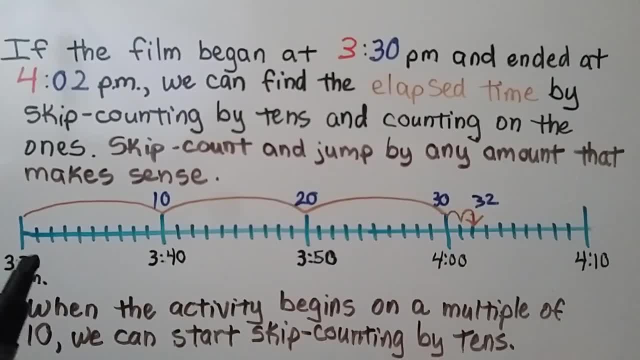 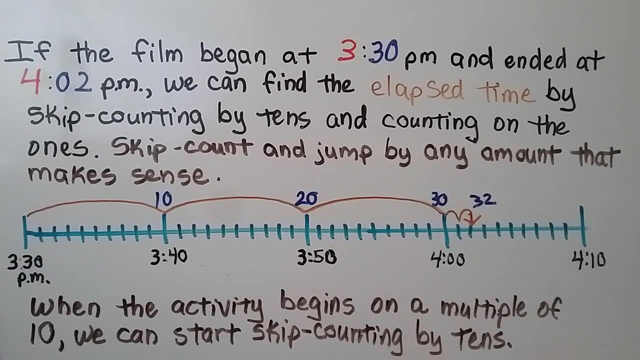 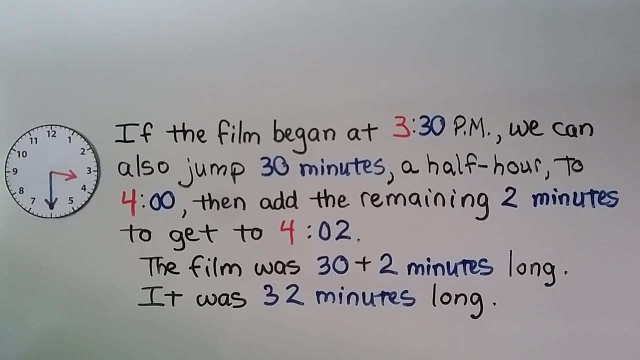 on our number line and our number line is going to depend on our number line on what the start minutes are. okay, if it said 35, then we could skip count by increments of 5. see, if the film began at 3: 30 pm, we can also jump 30 minutes. 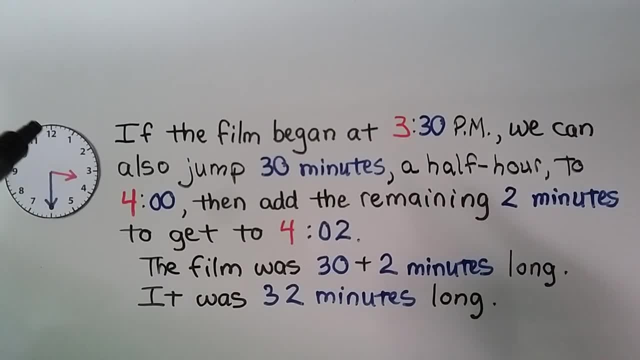 that's a half hour to 4 o'clock. when the minute hand finishes going around and it goes up to the 12 will be at 4 o'clock. that's a half hour. that's 30 minutes. so we can just jump 30 minutes. that half hour to four o'clock then add: 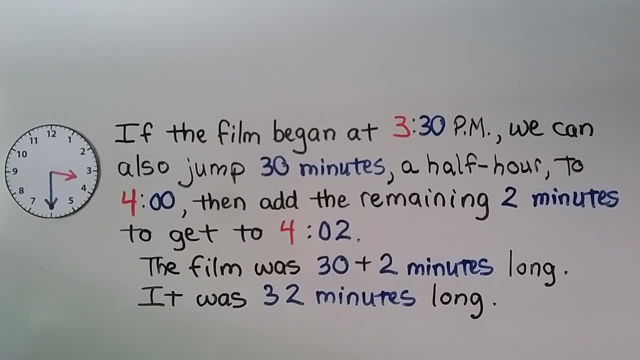 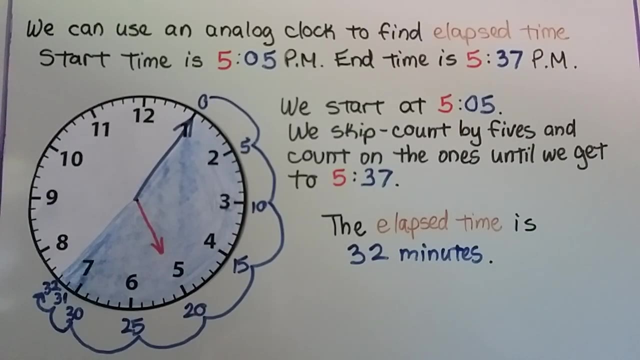 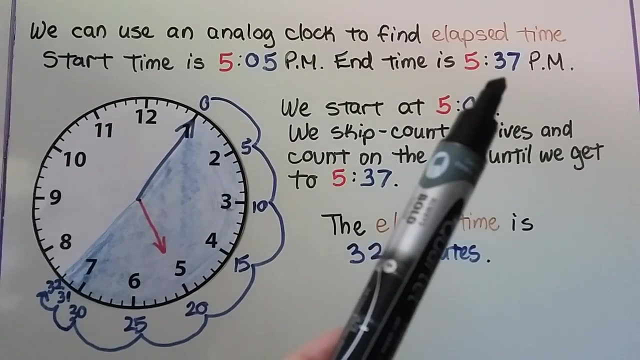 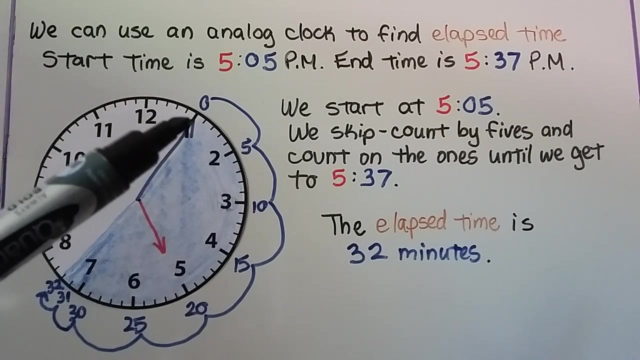 the two remaining minutes to get to 402 and the 30 minutes plus the two little minutes long, it was 32 minutes long. we can use an analog clock to find elapsed time. the start time is 505 pm. the end time is 537 pm. we start at 505 because it's the minute hands pointing on the one, so that's five. 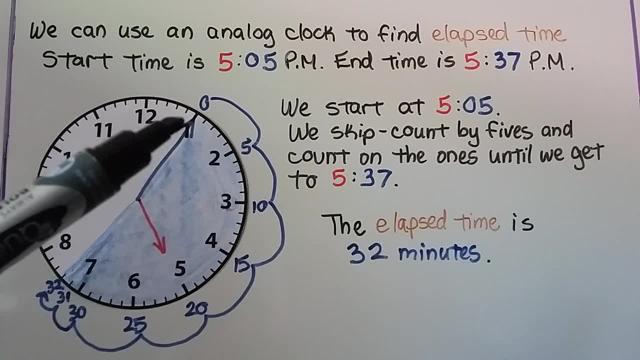 minutes past five, isn't it? and we skip count by fives, so that's going to end up becoming our zero mark, because that's the time that we're going to start counting. so that's going to end up becoming our zero mark, because that's the time that we're going to start counting. so that's going to end up. 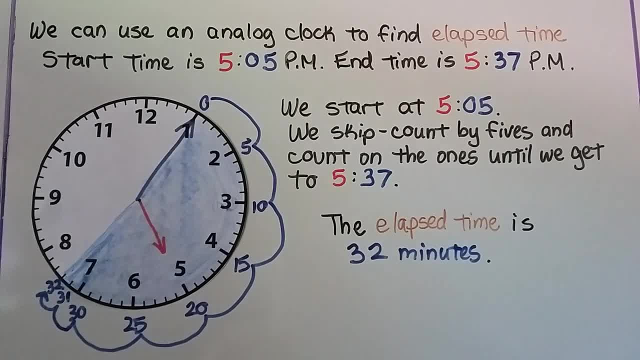 five minutes. see, we skip count by fives and count on the ones until we get to 537. so, starting here, the elapsed time would be 5, 10, 15, 20, 25, 30, 31, 32. so when it gets to 537, right here the elapsed 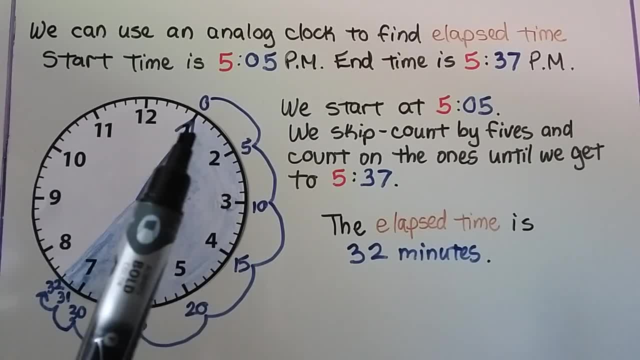 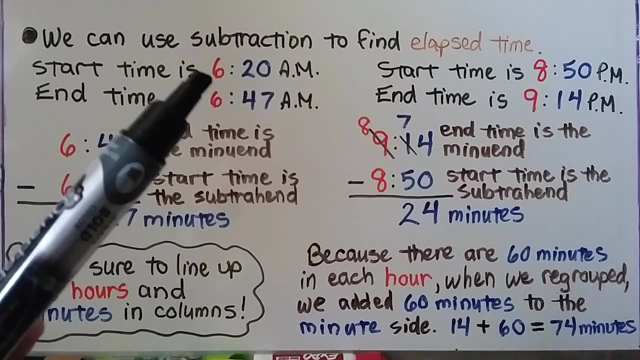 time would be 32 minutes. it's where the minute hand slowly moved around till it pointed to this little mark. we can use subtraction to find elapsed time. if our start time is 620 am and our end time is 647 am, we put the end time as the. 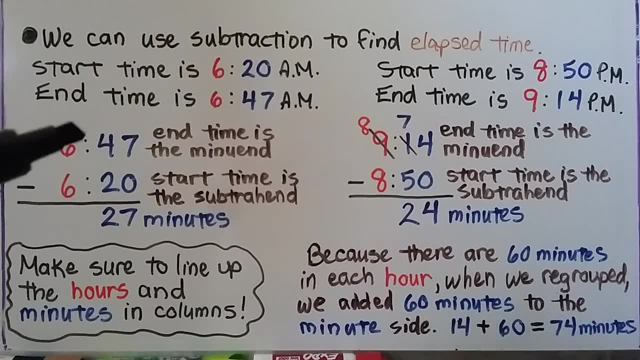 minu end. see how it went up on top. then the start time is the subtrah and we do our subtraction 7, take away zero is 7. then we do subtraction 7, take away zero is 7. then we do subtraction 7, take away 0 is 7. then we do subtraction 7, take away zero is 7. 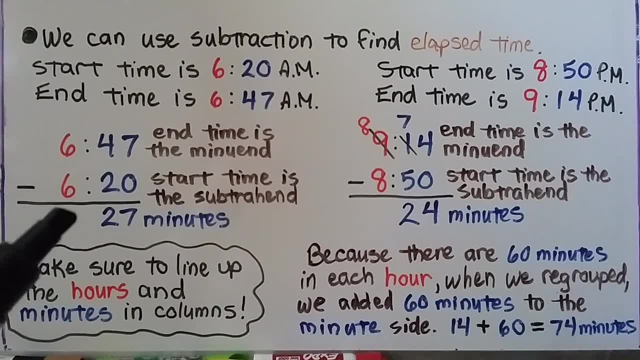 7,, 4 take away, 2 is 2,, 6 take away, 6 is 0, and we have 27 minutes. Just make sure to line up the hours and minutes in columns correctly and neatly, okay. Now this one's a little trickier. 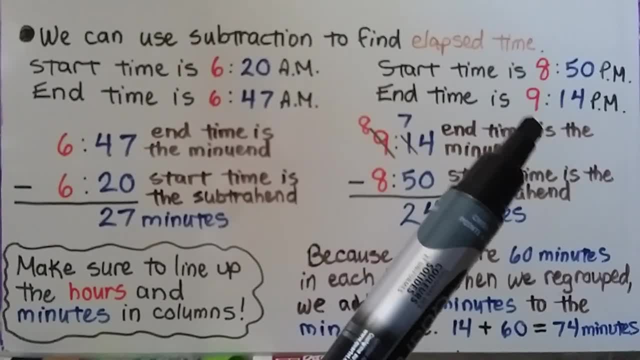 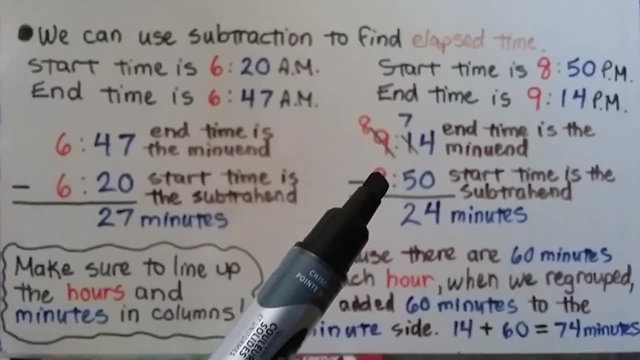 The start time is 8.50 pm and the end time is 9.14 pm. We put the end time as the minuend 9.14.. We put the start time as the subtrahend the 8.50.. 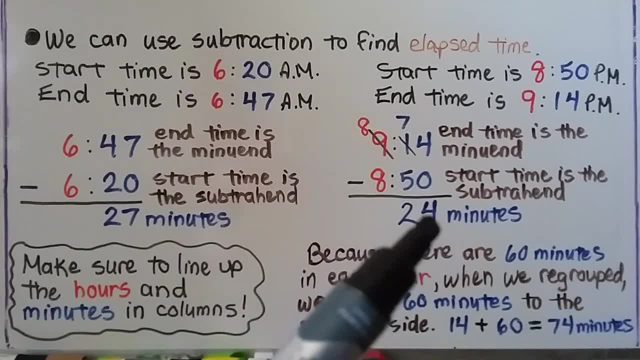 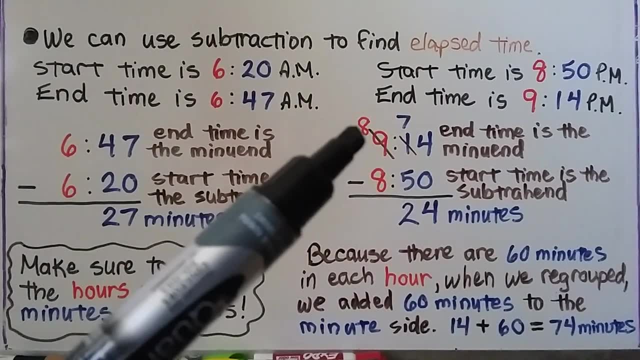 But we can do 4 take away. 0 is 4, but we can't have 1 take away 5.. So we need to regroup and borrow from the hours. So the 9 hours is going to become an 8 hours. 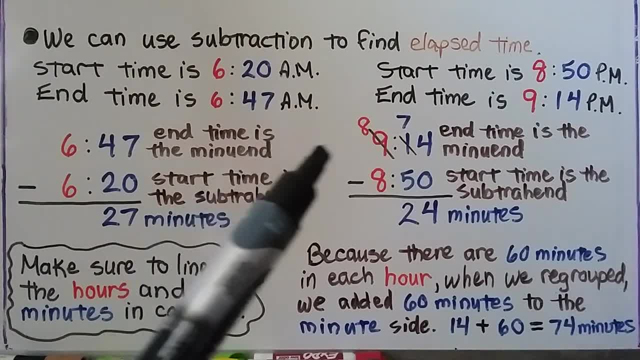 But each hour is 60 minutes. So if we take 60 minutes as an hour from here, we have to add 60 minutes to the minutes side, Because there are 60 minutes in each hour. when we regrouped, we added 60 minutes to. 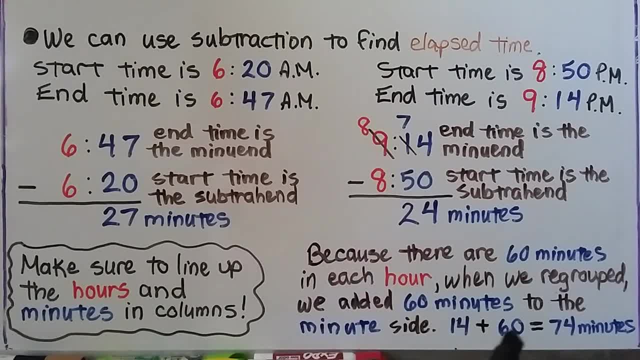 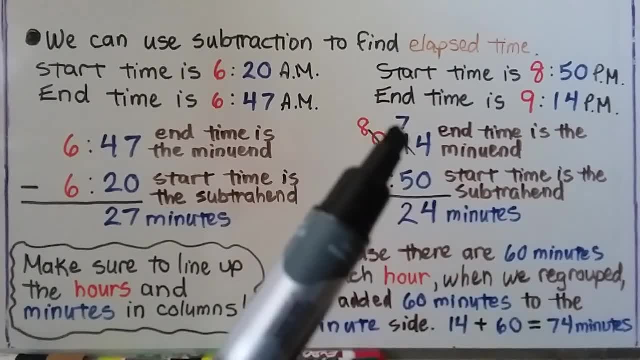 the minutes side, So we have 14 minutes. If we add the 60 minutes as the hour, we borrowed from the 9 and it became an 8, we now have 74 minutes. We have a 7 and a 4, see. 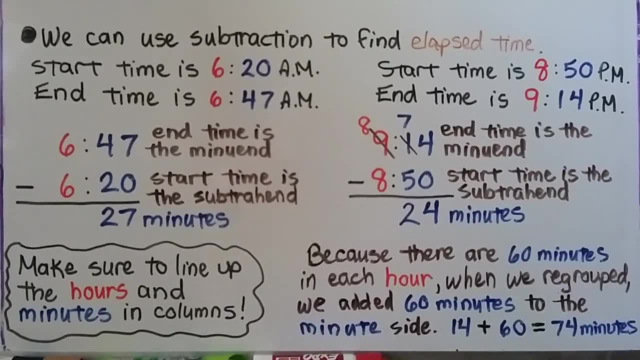 Now we can do the subtraction and do: 7 minus 5 is 2.. So that's a little trickier. We're going to get into that more in 5th grade, but I just wanted to show you what would happen. And it might even be easier to do this using a number line. 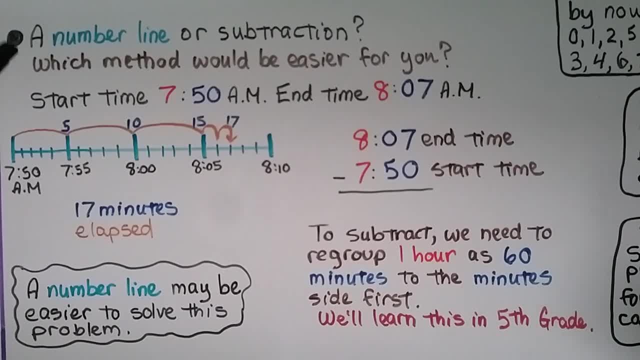 So let's talk about that a little bit more. A number line or a subtraction? which method would be easier for you? Our start time is at 7.50 am. Our end time is at 8.07 am. We use a number line. 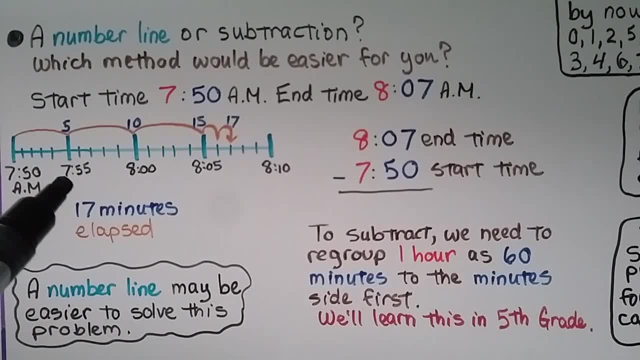 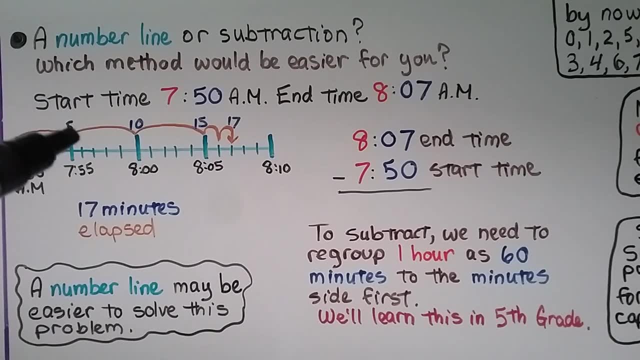 We can start at 7.50 and do increments of 5 to 7.55, then 8 o'clock, then 8.05 to 8.10.. Then when we skip, count by fives, 5,, 10,, 15,, we're at 8.05 for 15 minutes. 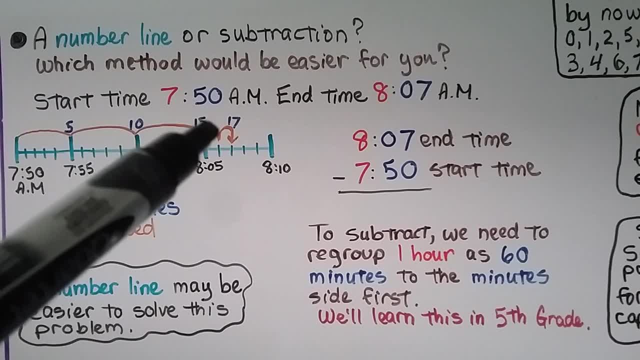 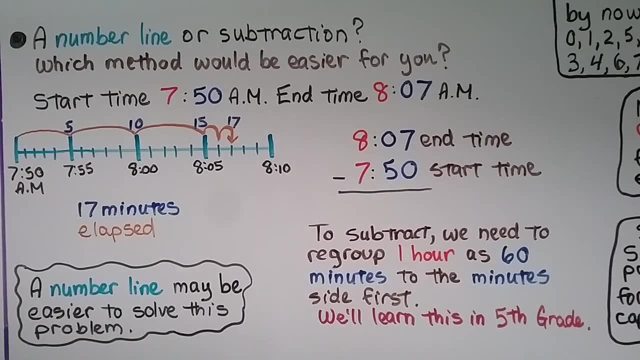 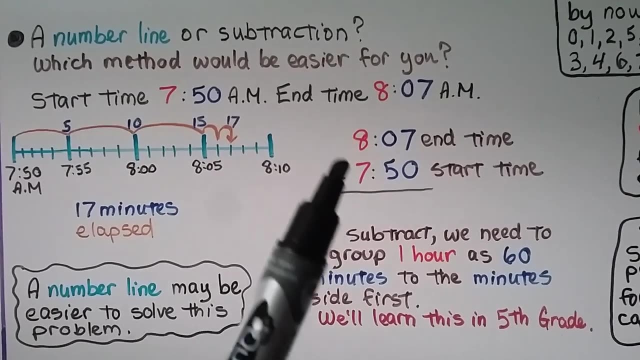 We need to get to 8.07.. So we can count on one that's 16 minutes and one more would be 17 minutes and we'd be at 8.07.. So we know 17 minutes elapsed. If we try doing it with subtraction, we put our end time as the minuend and our start. 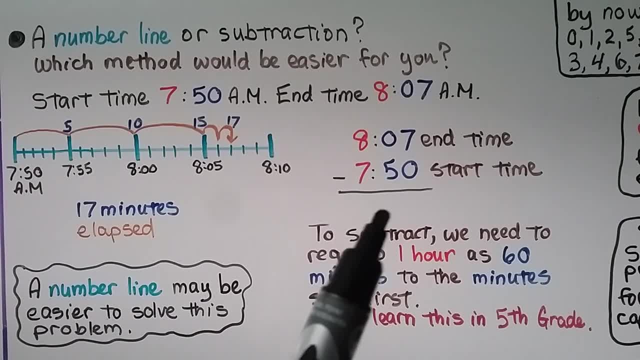 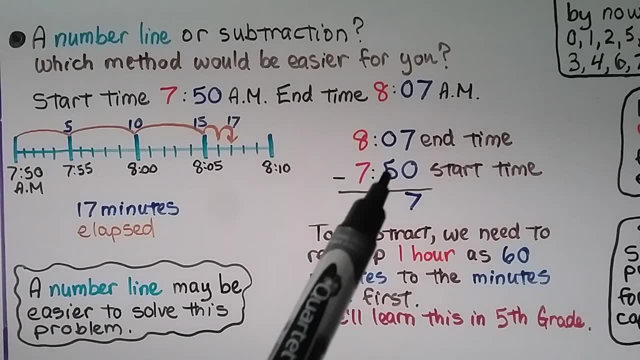 time as the subtrahend And we're back to likelihood, Back to like we had with the previous problem. We can do 7 take away. 0 is 7.. But now we have 0 minutes take away 5.. We need to regroup from the hours. 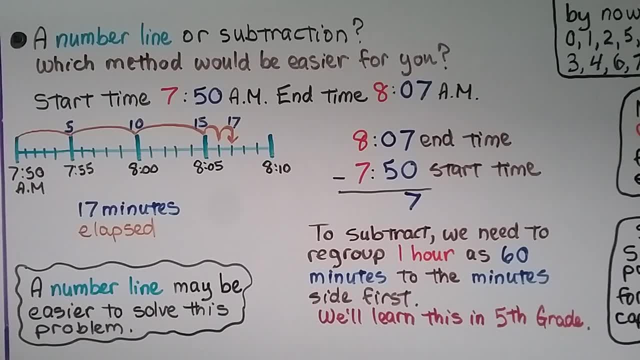 So we're going to cross off the 8 and make it a 7. And we're going to take the 60 minutes from that hour that we're borrowing and we're going to give it to the minutes side. So we gave 60 minutes to the minutes side. 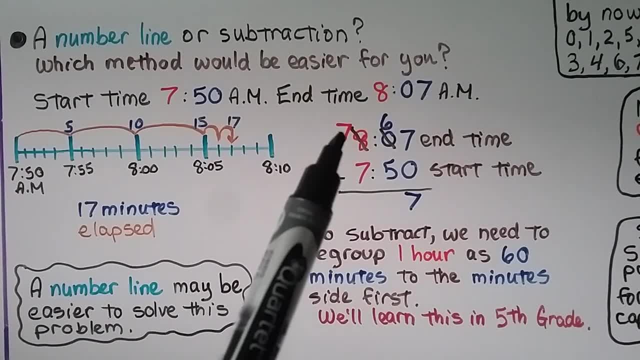 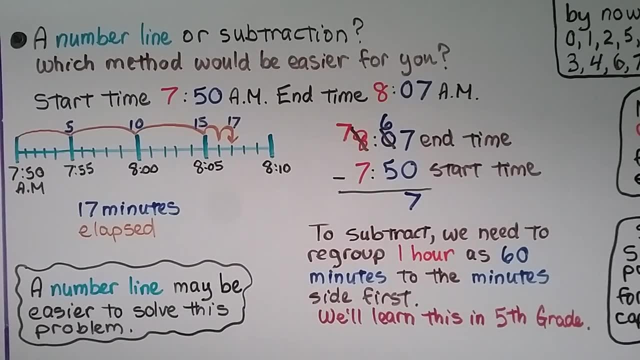 We had 7 minutes. we borrowed 60 minutes as an hour. now we have 67 minutes on the minutes side And 6 take away. 5 is 1 and we get 17 minutes, just like we did with the number line. 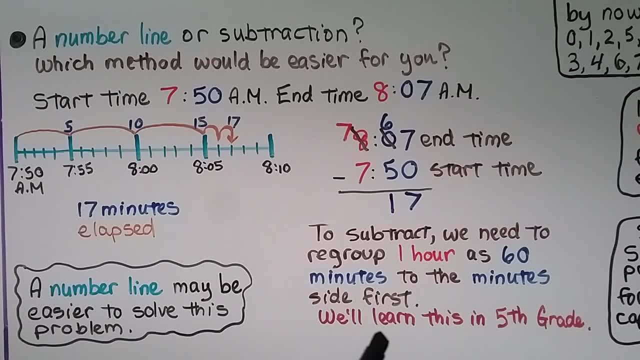 So to subtract, we need to regroup one hour as 60 minutes to the minutes side first. We're going to learn more about this in 5th grade, But a number line may be easier to solve this problem right now for 3rd grade. 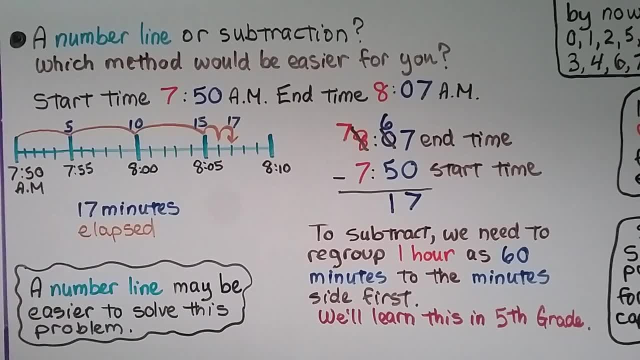 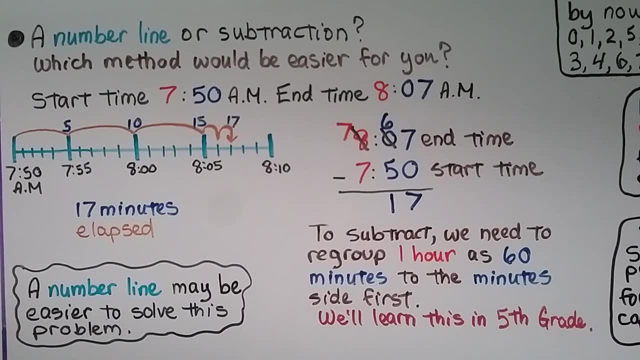 We can see the increments and not have to worry about regrouping. If you know how to regroup this and you understood this well, then good for you. you're ahead of the class. But if this is too difficult, don't worry about it. 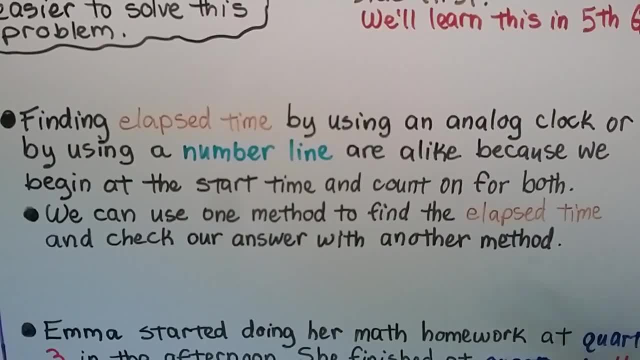 You're going to learn it in 5th grade- And finding elapsed time by using an analog clock or by using a number line are alike, Because we begin at the start time and count on for both, We can use one method to find the elapsed time. 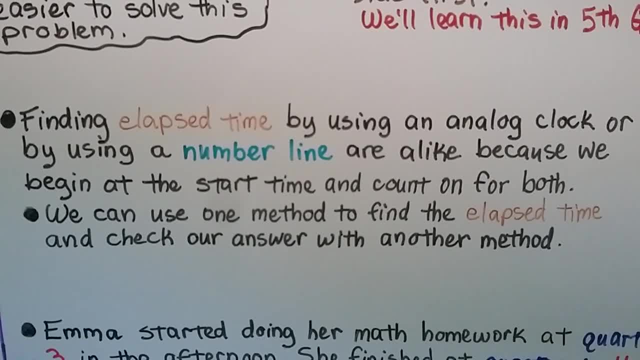 And check our answer with the other method. If we use a number line and find our elapsed time, we can check it by using a drawing of an analog clock. If we find the elapsed time using an analog clock, we can check it using the number line. 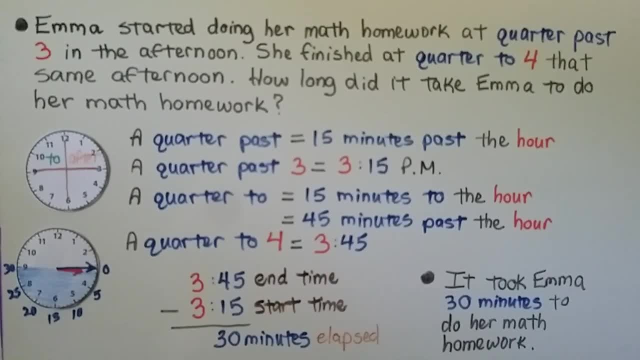 Emma started doing her math homework at quarter past 3 in the afternoon. She finished at quarter to 4. That same afternoon. How long did it take Emma to do her math homework? Well, remember that a clock can be split into quarters. This is a quarter after. 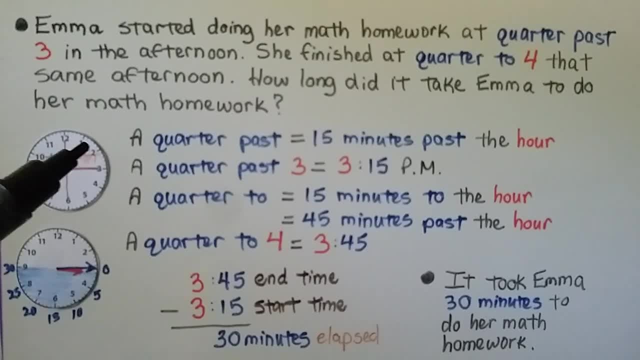 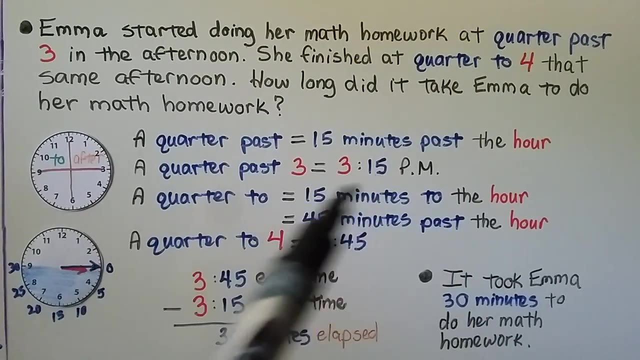 This is a quarter to A quarter. after is a quarter past and it's 5, 10,, 15 minutes past the hour. So a quarter past 3, that's when she started. quarter past 3, that would be 3, 15.. 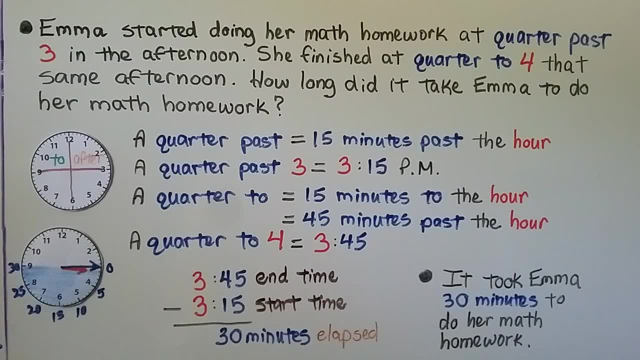 The minute hand 10 would be pointing to the 3 and that stands for 15 minutes. It would be 3, 15 pm. A quarter to is equal to 15 minutes to the hour or before the hour. It's also 45 minutes past the hour. 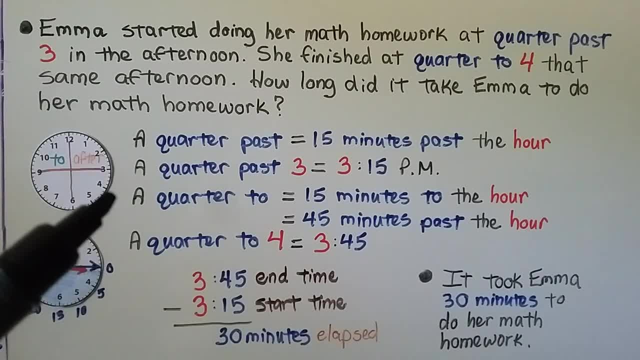 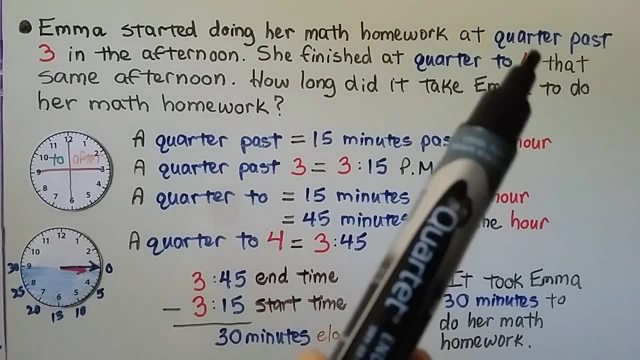 We can start at 12 as a zero and go 5,, 10,, 15,, 20,, 25,, 30,, 35,, 40,, 45. It's not 4 o'clock yet, It's a quarter to 4.. 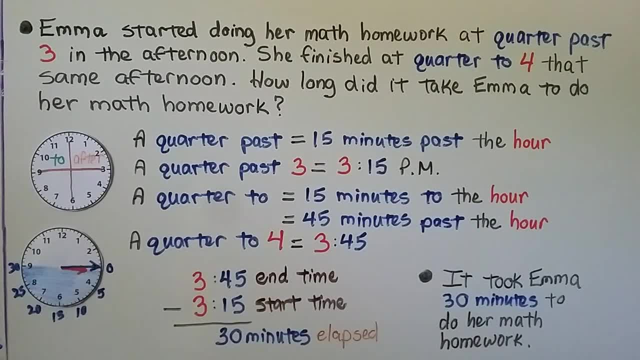 So that means it's 15 minutes before the hour, 15 minutes before 4 o'clock, So it's still in the threes. The hour is still in the threes. So a quarter to 4 would be 3, 45 pm. 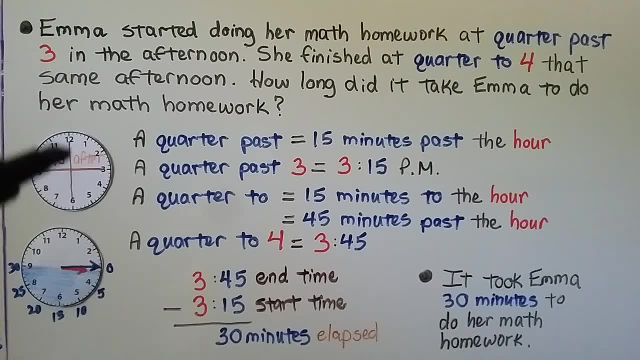 It's not 4 o'clock yet, So it's still in the threes. And if we skip count by fives going around, the 9 is a 45. That's 3, 45. So we have 3, 45 for our end time using subtraction. 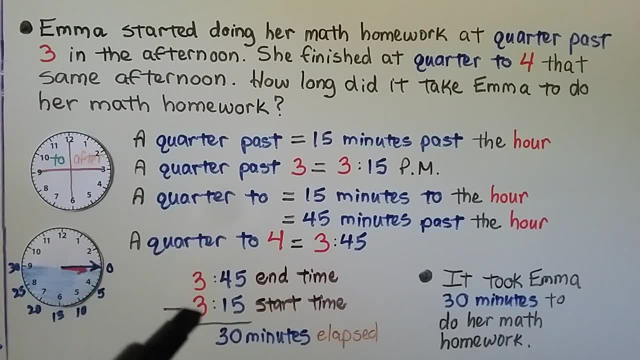 The end time is the minuend And we put 3, 15 for our start time as the subtrahend. We do our subtraction and get 30 minutes elapsed. The clock was at 3, 15 and 5,, 10,, 15,, 20,, 25, 30 minutes elapsed. 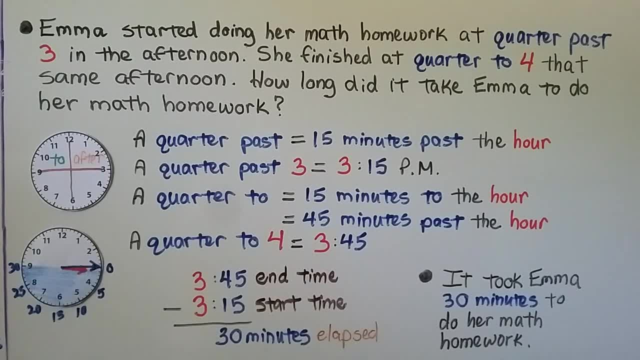 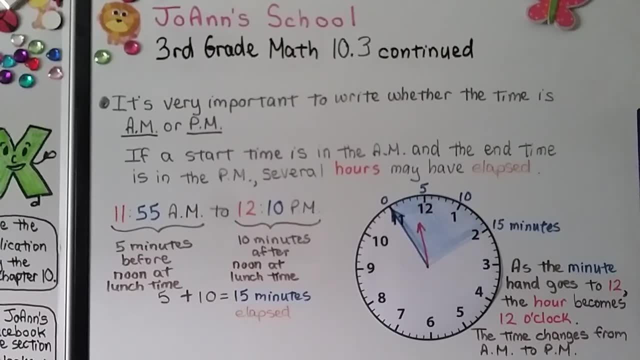 So it took Emma 30 minutes to do her math homework. It's very important to write whether the time is am or pm. If a start time is in the am and the end time is in the pm, several hours may have elapsed. 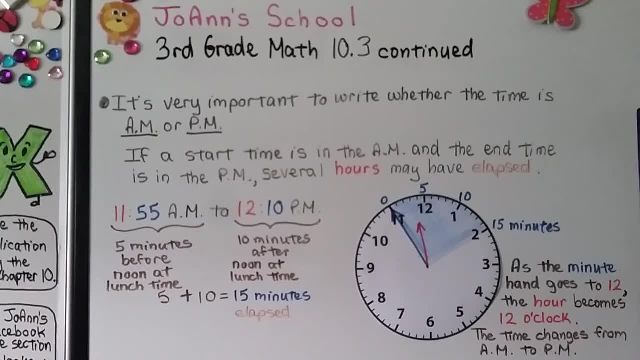 It might be a few minutes, like I'm going to show you in this example, but it also might be hours, If we start at 11, 55 am and go to 12, 10 pm. this is 11, 55 am. It's not 12 o'clock yet, but it's almost. In five more minutes it'll be 12 o'clock, And we start at 11, 55 am And go to 12, 10 pm, And then it goes to 12, 10.. 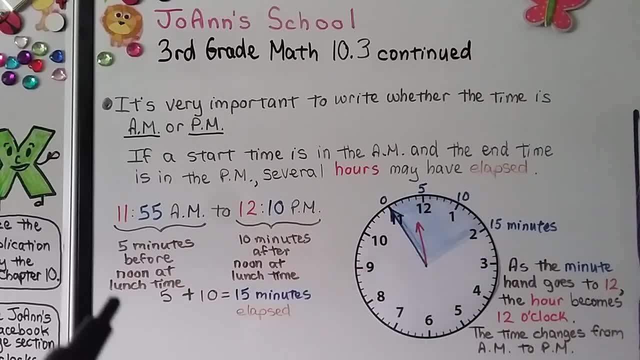 So we have 5,, 10,, 15 minutes. This is 5 minutes before noon at lunchtime. This is 10 minutes after noon at lunchtime. So the 5 minutes before noon and the 10 minutes after is 15 minutes elapsed. 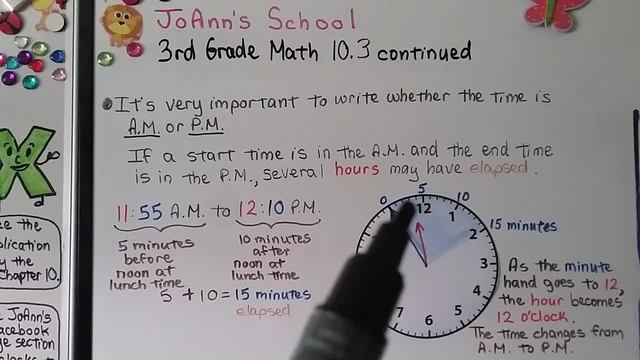 As the minute end goes to the 12, the hour becomes 12 o'clock. It becomes 12 o'clock noon at lunchtime And the time changes from am to pm. So we just have 15 little minutes that the minute hand moved. 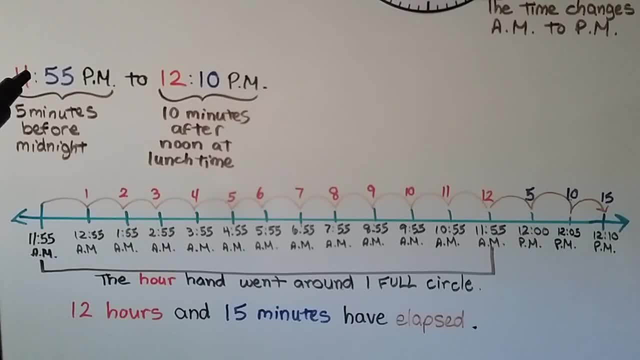 If we start at 11, 55 pm and go to 12, 10 pm, this is 5 minutes before midnight. This is 10 minutes after noon at lunchtime. So you have to be very careful when we're writing our time. 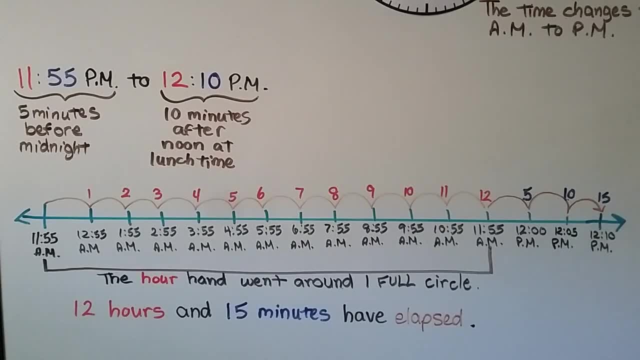 We need to write am or pm so we know how much time has elapsed And if we're counting nights or days, If we make a number line going from 5 minutes before midnight at 11, 55 pm. 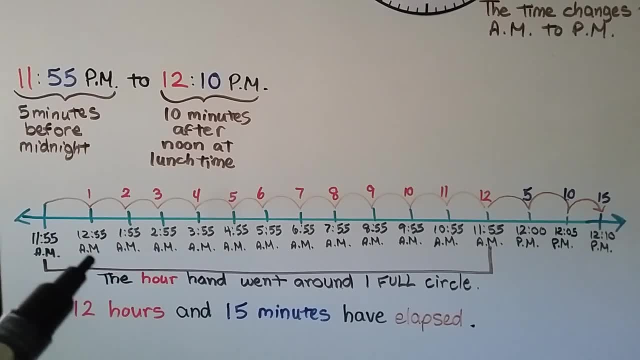 1 hour would be 12, 55 am, Because now it's morning. We went from the middle of the night to now it's after midnight, So it's 12, 55 am. So that would be 1 hour to 12, 55,, 2 hours to 1, 55.. 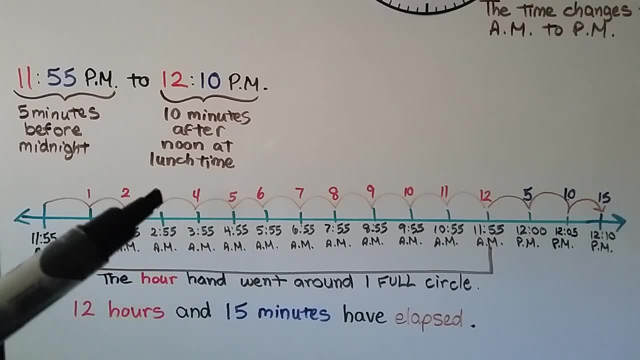 And we just keep going to the 55 on the clock. So we got 3,, 4,, 5,, 6,, 7,, 8,, 9,, 10,, 11,, 12 hours to get back to 11, 55 am. 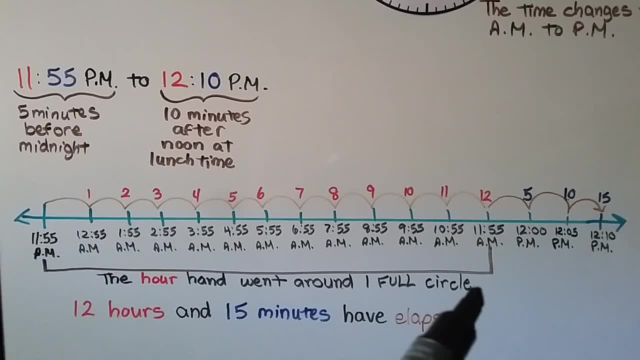 Because the hour hand went around one full circle. It went around 12 hours, So it went from 11, 55 pm to 11, 55 am. We need to go to 12, 10 pm. 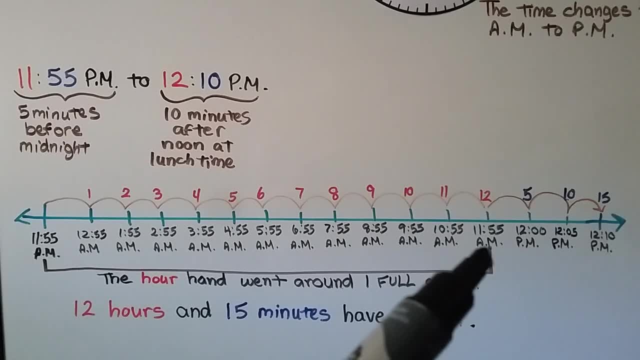 5 more minutes. it's going to be 12 o'clock. It'll be 12 o'clock noon at lunchtime. See Then. another 5 minutes is 12, 05, and another 5 minutes is 12, 10 pm. 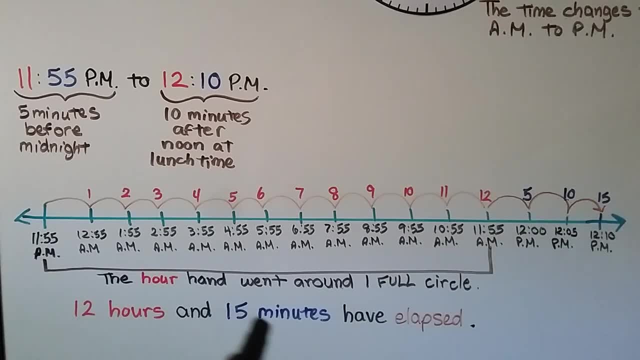 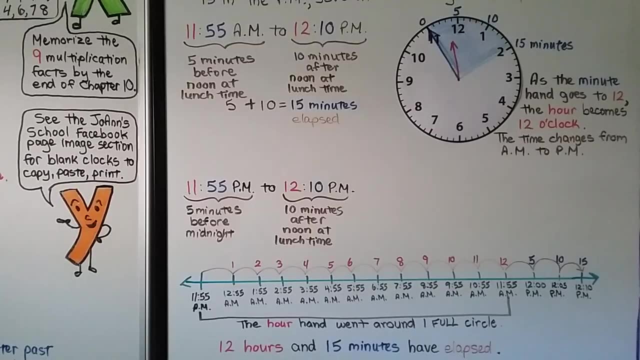 So we went 12 hours and 15 minutes. 12 hours and 15 minutes have elapsed because this says pm and that says pm, Because this says am and that says pm. only 15 minutes elapsed When we made it pm and pm the clock hand. 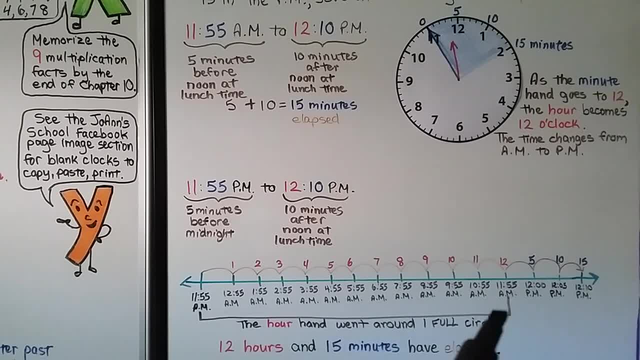 the minute hand had to go one full circle around the clock to go back to 11, 55 am, And then we added on that 15 minutes. So we have 12 hours and 15 minutes that have elapsed. Be very careful and make sure you write am or pm. 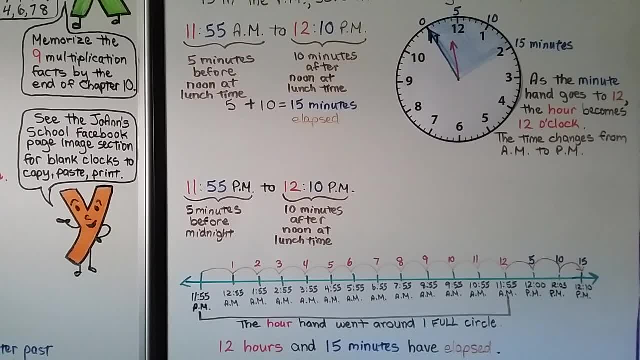 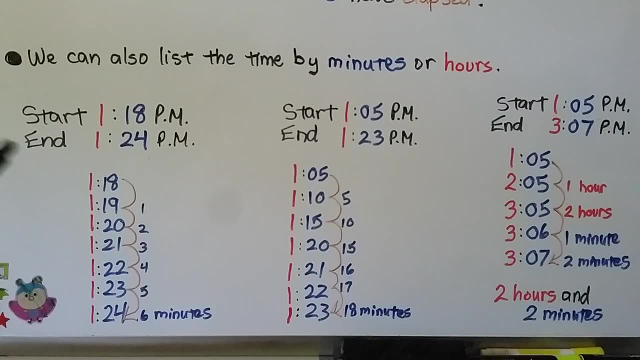 So it's not confusing whether you're talking about day or night. We can also list the time by minutes or hours. If our start time is 1, 18 pm and our end time is 1, 24 pm. 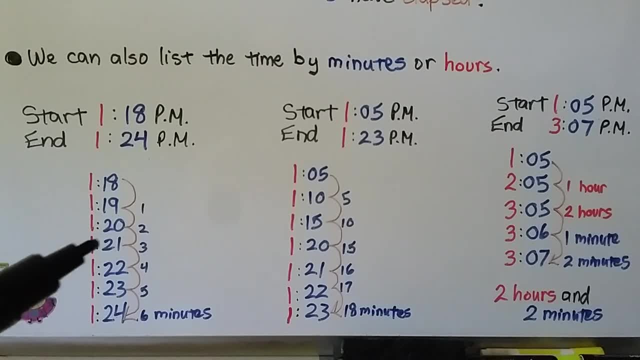 we can write 1, 18,, 1, 19,, 1, 20,, 1, 21,, 1, 22,, 1, 23,, 1, 24.. We start here and we count: 1 minute, 2 minutes, 3 minutes, 4 minutes, 5 minutes, 6 minutes. 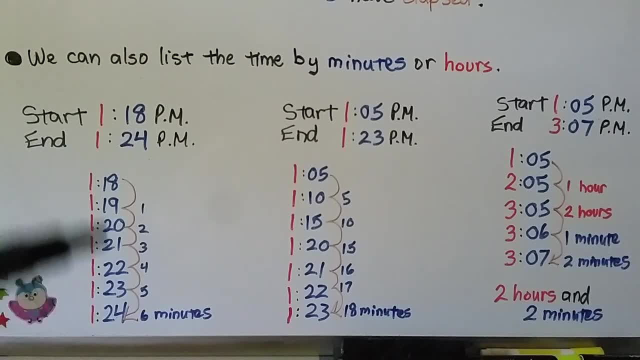 And it's the same thing as using a number line. We're just making it in a list going this way, instead of writing it on a number line with little marks going this way, If our start time is 1, 05 pm. 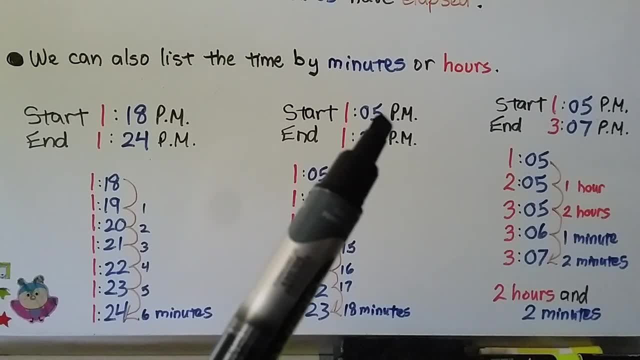 and our end time is 1, 23 pm. because that's a five, we can skip count by fives And we can write our start time of 1, 05, then write 1, 10,, 1, 15,, 1, 20,, 1, 21,, 1, 22,, 1, 23..